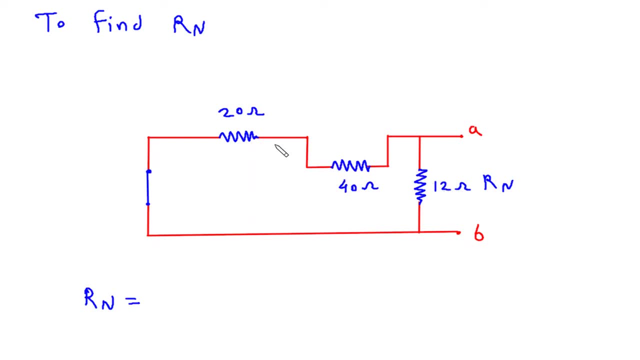 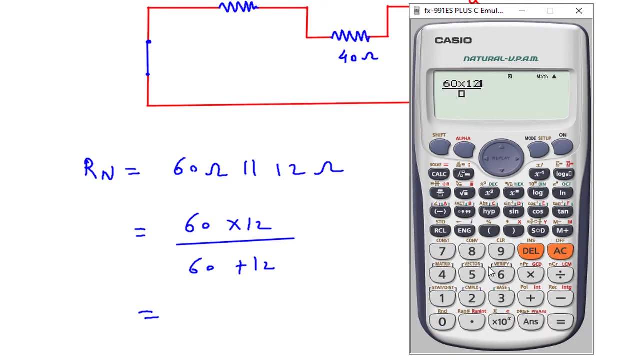 and it is in parallel with 12 ohm. So this will be 60 ohm parallel with 12 ohm, 60 ohm parallel with 12 ohm. So 60 into 12 divided by 60 plus 12.. 60 into 12 divided by 60 plus. 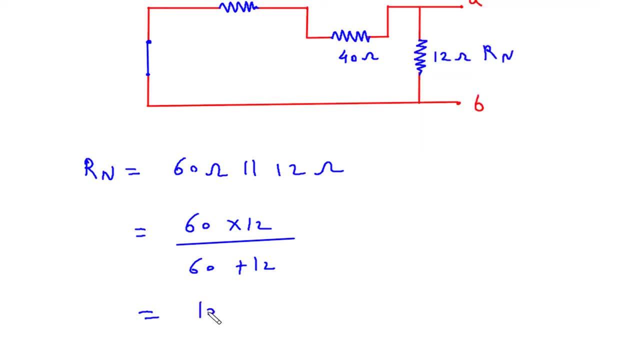 12.. So it is 10 ohm. Therefore Rn is equal to Norton's, resistance is equal to 10 ohm. Next we have to find In. To find In, we will short circuit the terminal AB. So this will be 12. 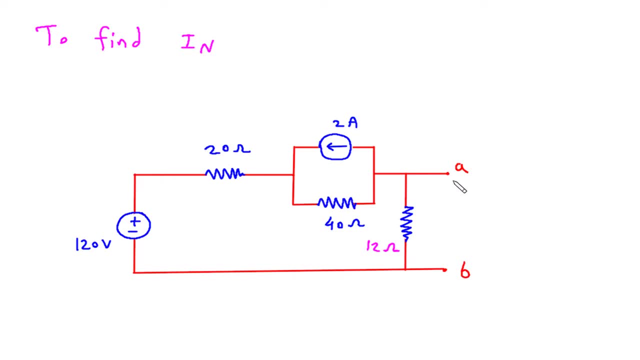 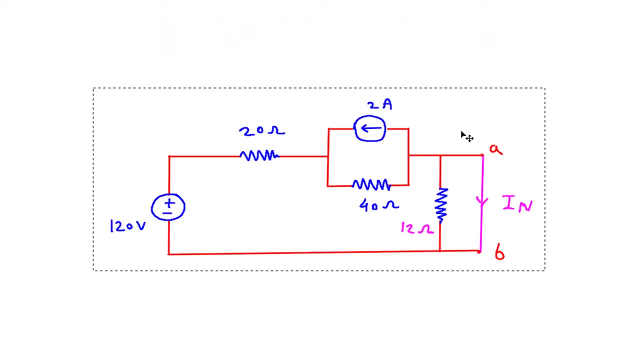 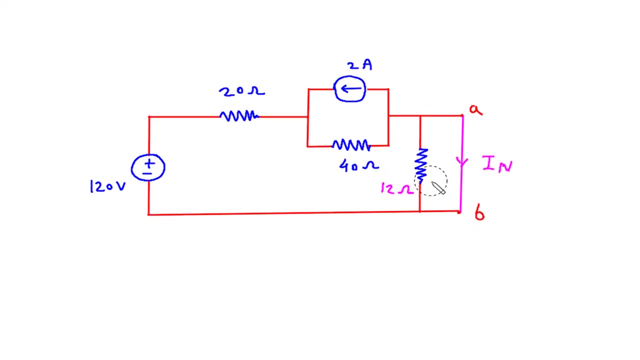 ohm. We will write it on left side. Now we will short circuit this terminal AB and this will be current In Now to find In. we will convert this 2 ampere current source into its equivalent voltage source. Also, as we can see that this 12 ohm is short circuited, So this will be: 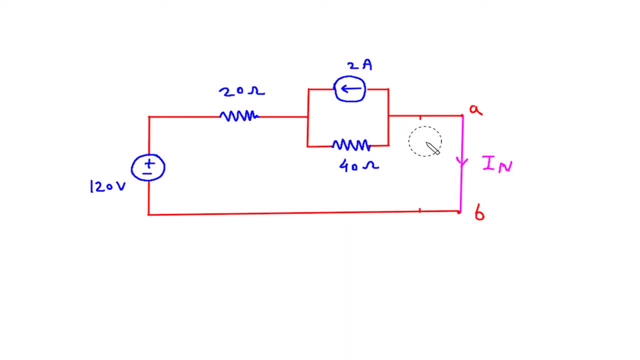